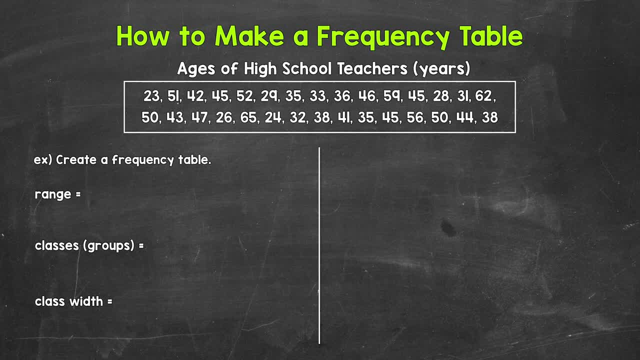 show us the number of times something occurs in a data set. Let's jump into our example and see how to make a frequency table to represent our data. So we have the ages of the teachers at a high school. Now the first thing that we need to do is find the range of the data. The 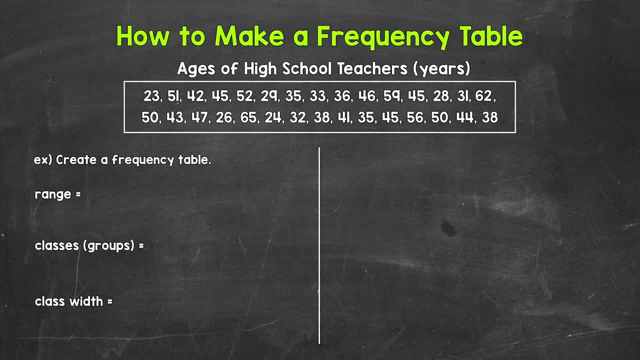 range tells us how far our data spans, so how spread out the data is between the highest, highest value and lowest value. Knowing the range will help us determine how we are going to approach making our table. It starts us off. All we need to do here is find our highest number. 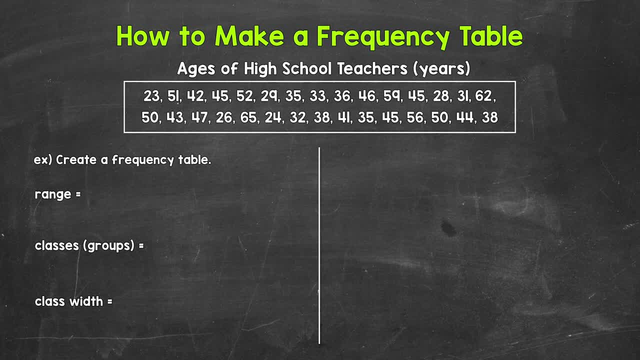 in value and lowest number in value. then find the difference between them. The highest number in value is 65, and then the lowest number in value is 25.. The oldest teacher is 65 and the youngest teacher is 23.. Let's find the difference. 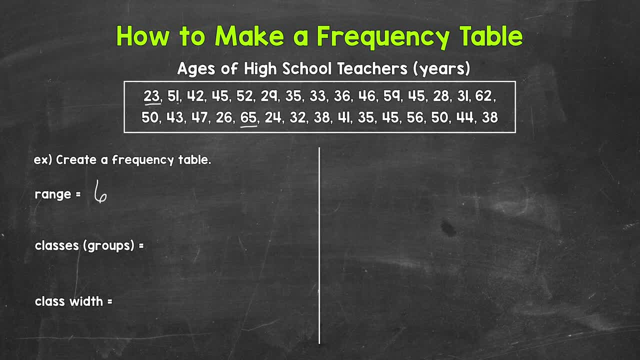 So we need to subtract. so let's do 65 minus 23.. 65 minus 23 gives us a range of 42. Seeing that our range is 42, we're not going to want to click on any of the values that be in the table, So let's just look at what we have here. I'm going to 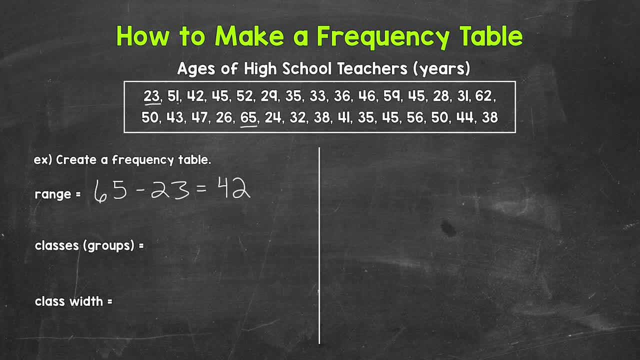 write each individual number within our table. We don't want to start at 23 and then count up to 65. That table would be extremely long and then also the frequency for each value, each age, would be only 1 or 0. We may have a 2 here or there. That would not be the best way to set. 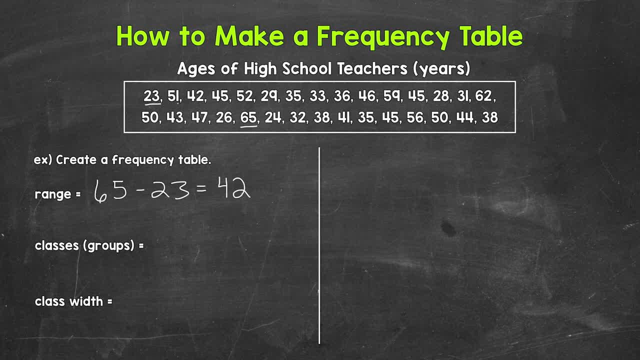 this table up. So we're going to make a grouped frequency table. We will have groups called classes or class intervals, that the ages will fall within. So the next thing we need to do is determine the number of classes, the number of groups we want. For this example, let's use 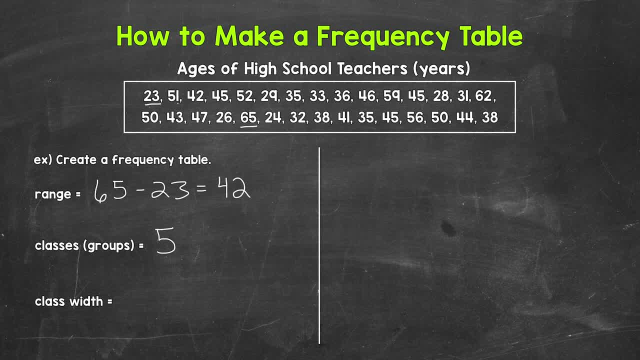 5 classes. This is going to be a good number for this data and set our table up nicely. As far as determining how many classes for a frequency table, typically speaking, there's going to be a number of classes that we want to set up, So we're going to set up a number of. 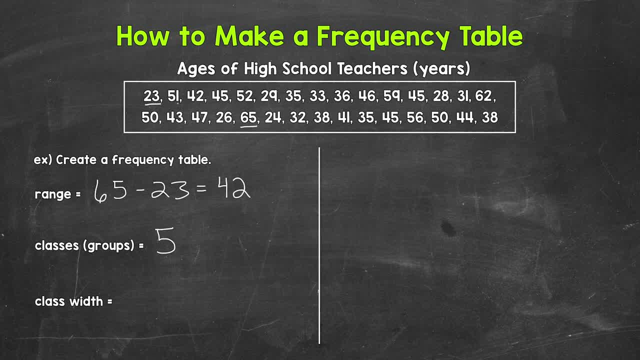 classes for a frequency table. So we're going to set up a number of classes for a frequency table, somewhere between 5 and 15 classes or 5 and 20 classes, And this depends on the data, the range of the data and how you want to set your table up. Again, for this example, 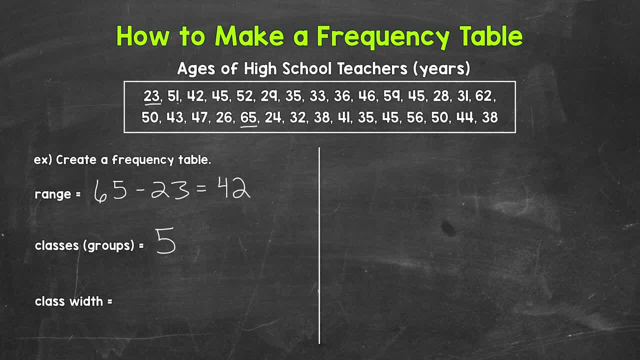 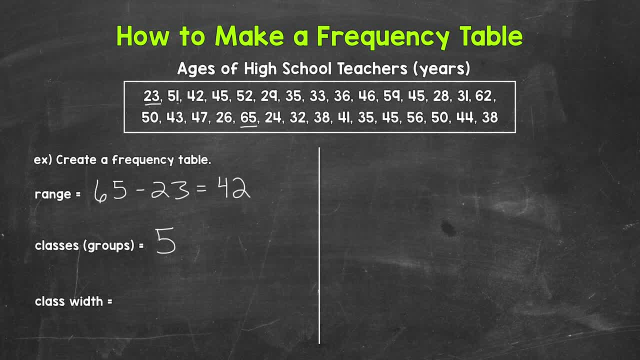 classes that we want to set up Again. for this example, we're going to set up a number of classes that we want to set up Again. for this example, we're going to set up a number of dividing it by the number of classes we want, So we can use this for our class width, or it will. 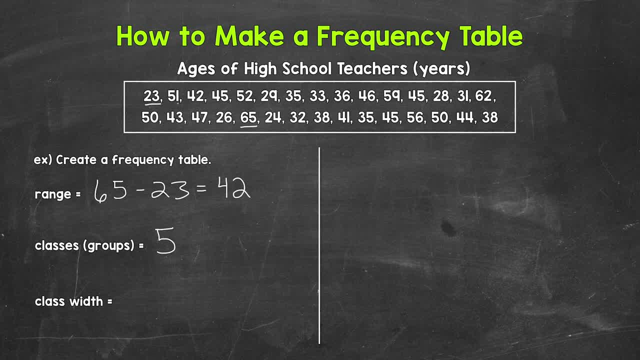 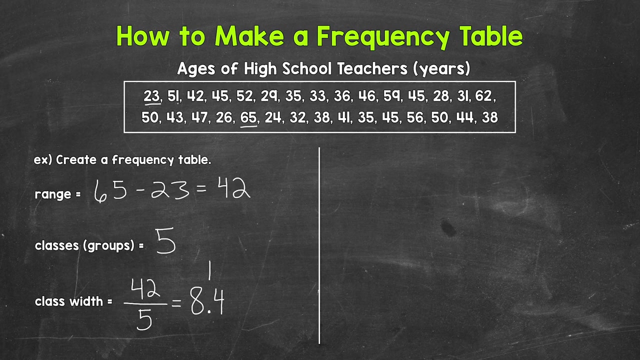 at least give us a starting point and something to go off of. Our range is 42, and then we want 5 classes, So let's do 42 divided by 5. That gives us 8 and 4 tenths. Once we have this, we always round up 8, and 4 tenths rounds up to 9.. This number gives us an 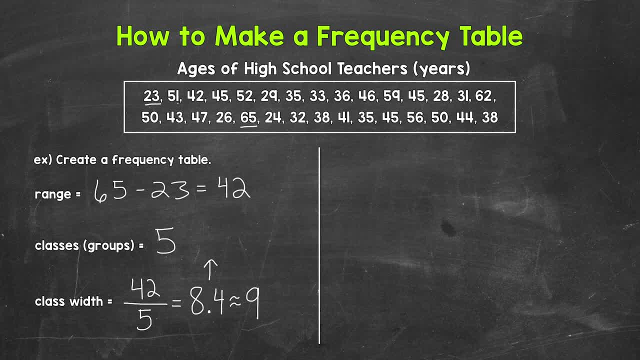 idea for our class width. Now, we can absolutely use 9, but we're actually going to round all the way up to 10 and use 10 for our class width. So let's use 10.. This is because we are working with ages. 10 makes more sense. 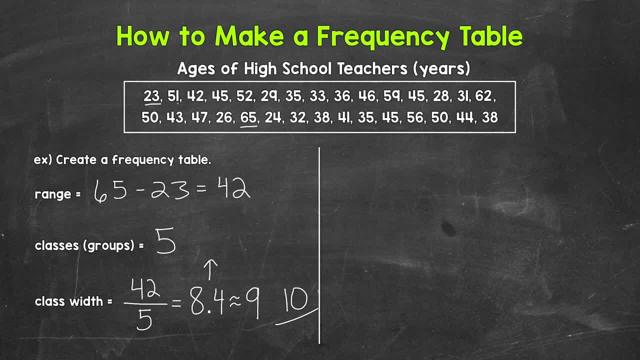 10 is kind of a natural group for ages. It will be more convenient and work better for our table. That way we have the 20s, the 30s, the 40s, the 50s and the 60s. 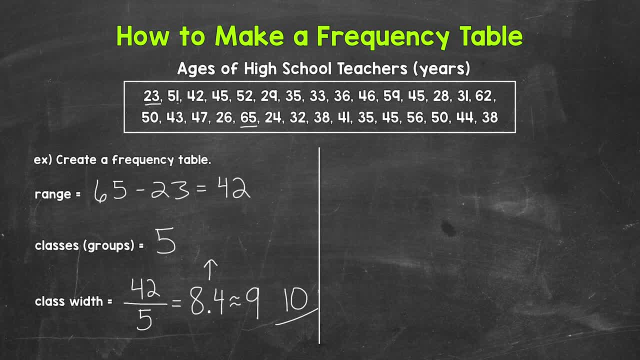 So just to recap here as far as class width, we took the range 42 and divided it by the number of classes 5. That gave us 8 and 4 tenths. We always round that up. So we rounded 8 and 4 tenths up to 9.. Now again, can we make a frequency table using 9 for the? 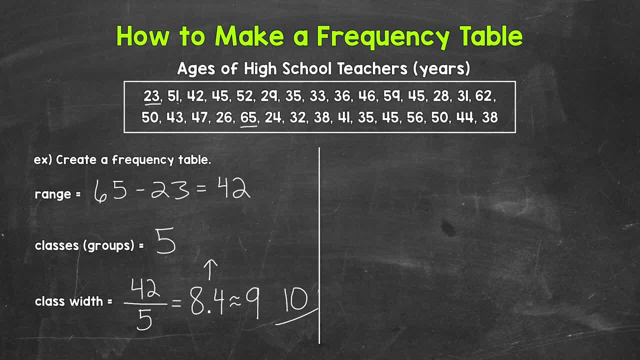 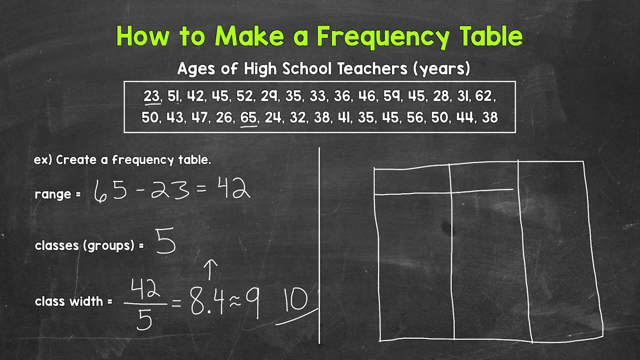 class width: Absolutely, But we're using 10 because that makes a little more sense for the ages, The data we are working with. Now we can start our table. We will make three columns And then a row up top for our column headers, The labels. The column on the left will be the ages column. 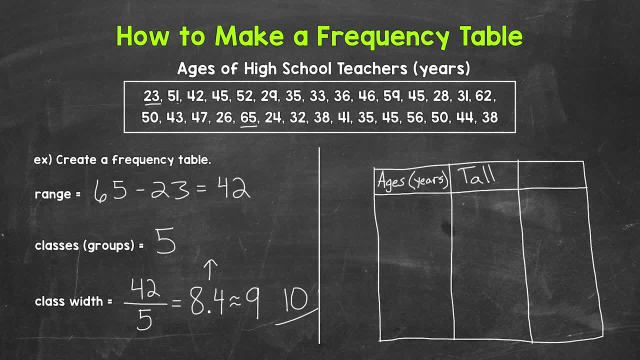 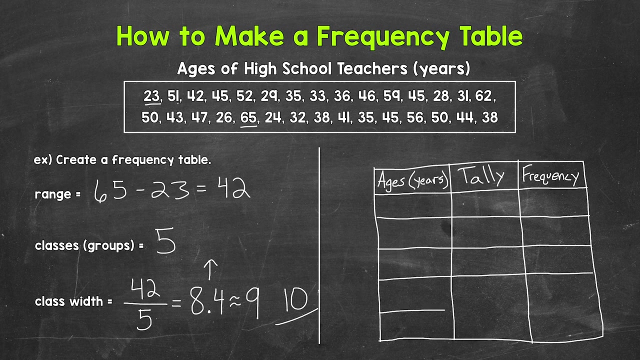 The middle column will be the tally column, And then the column on the right will be the frequency column. Now we need five more rows. Five rows, rows for our classes. So 1,, 2,, 3,, 4, and 5.. Now we can fill in our classes, The first thing that we 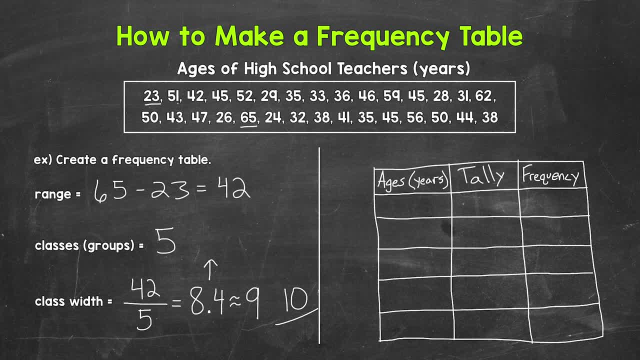 need to do, though, is determine our starting point. We can either start with our lowest number in value, which is 23, or something a little under that. We need to make sure all of the data is included. Let's start a little under 23.. So let's start with 20.. This will give us nice classes to 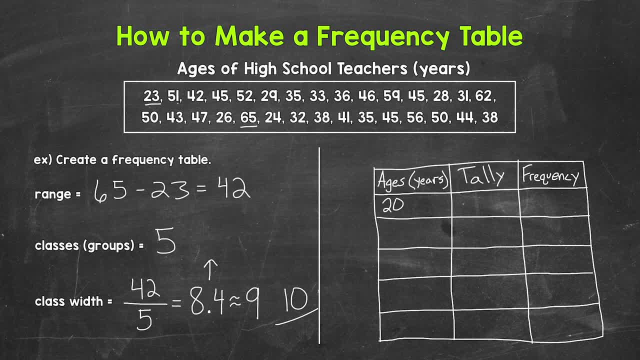 work with and classes that make sense for our table. Remember, our class width is 10.. So this first class is 20 to 20.. Now you may be thinking 20 to 29 is only a class width of 9, but actually it is 10.. The class width: 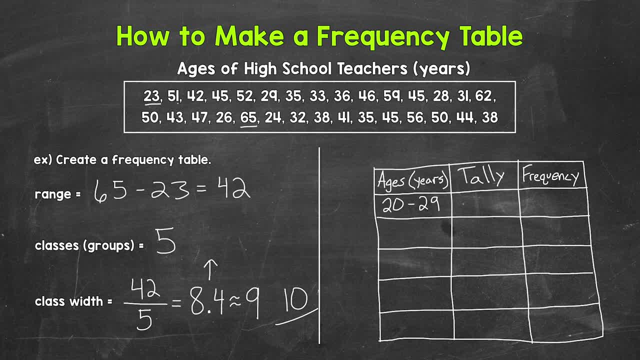 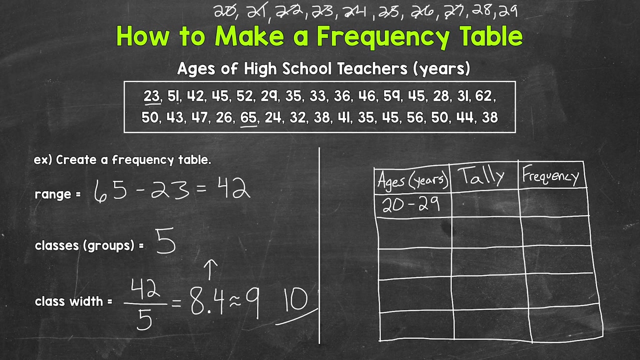 is how many numbers we have within a class, a group. Think about it. We do have 10 numbers here. I'll write them out up top: 25,, 26,, 27,, 28,, 29.. 1,, 2,, 3,, 4,, 5,, 6,, 7,, 8,, 9,, 10.. So our class width is 10 there. So that's. 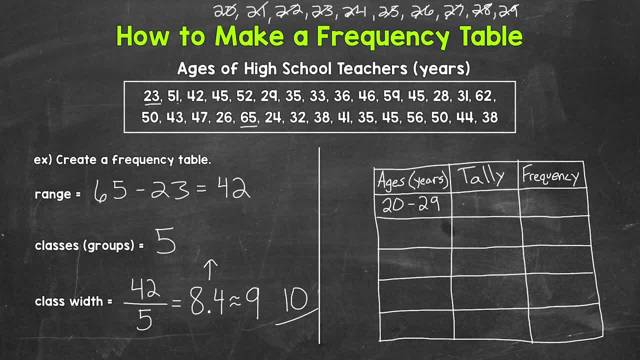 something to keep in mind and be careful with. After 20 to 29 years old, we have 30 to 39 years old, Then we have 40 to 49 years old, Then 50 to 59 years old And then 60 to 69 years. 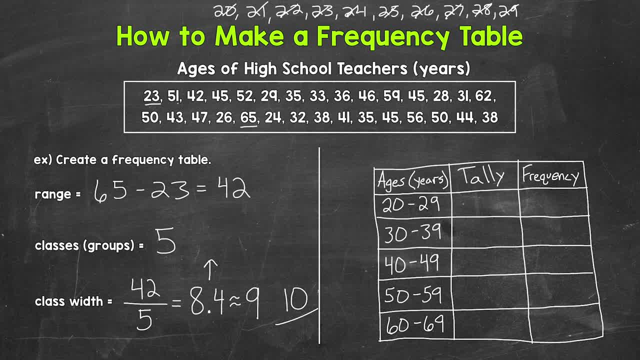 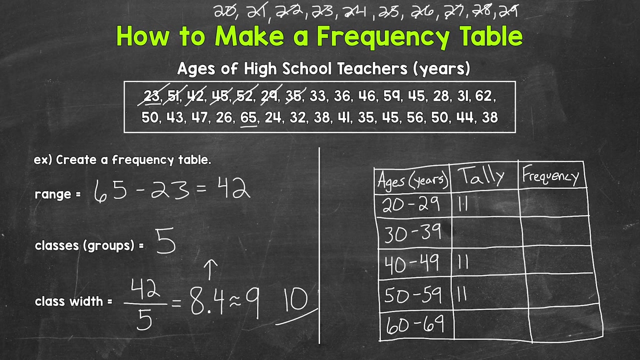 old. So those are our five classes. Now we can work through our data and tally everything up. We will work from left to right and put a tally in the correct group for each of our classes. Let's start with 23.. So 23 goes right here. Then we have 51,, 42,, 45,, 52,, 29,, 35,, 33,, 36,. 46,, 59,, 45,, 28,, 31,, 62,, 50,, 43,, 47,, 26,, 65,, 70,, 62,, 80,, 91,, 92,, 93,, 93,, 94,, 93,, 94,. 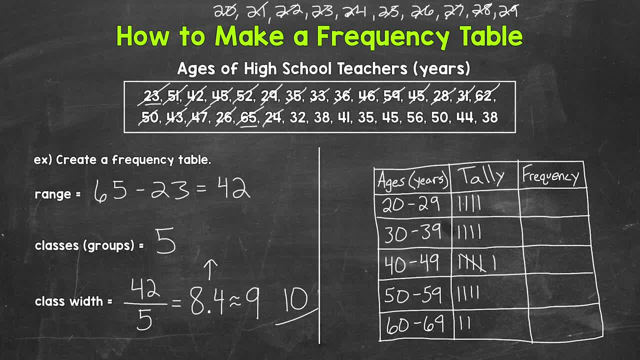 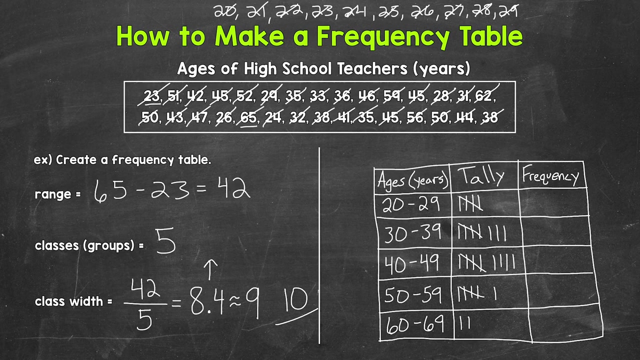 24,, 32,, 38,, 41,, 35,, 45,, 56,, 50,, 44,, 38.. Lastly, let's count everything up and put the final frequency for each age group. Let's start with 20 to 29 years old.